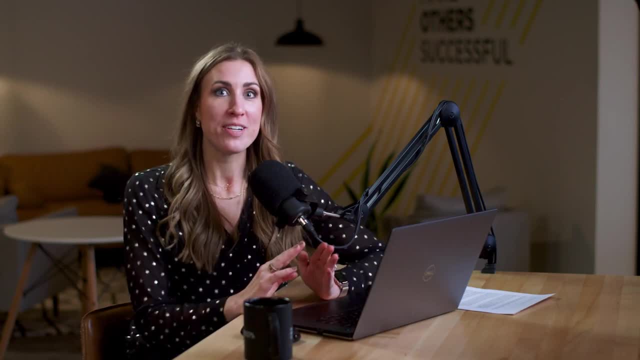 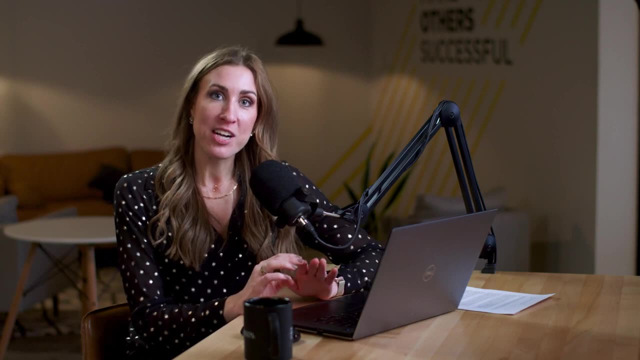 getting asked questions such as: when is the best time to start a project? When is the best time to start a project? When is this due? What tasks are assigned to me? Where can I get updates? Where can I find documentation or meeting minutes? By putting projects into Teams, you have a central channel. 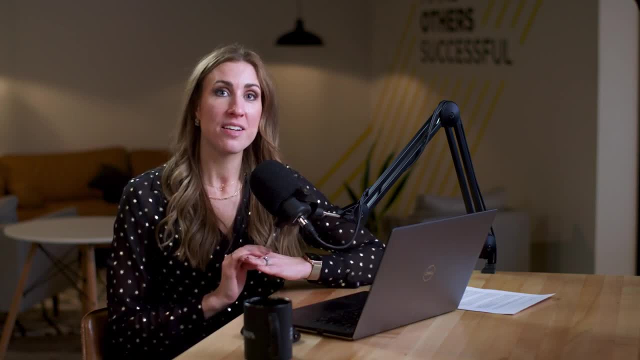 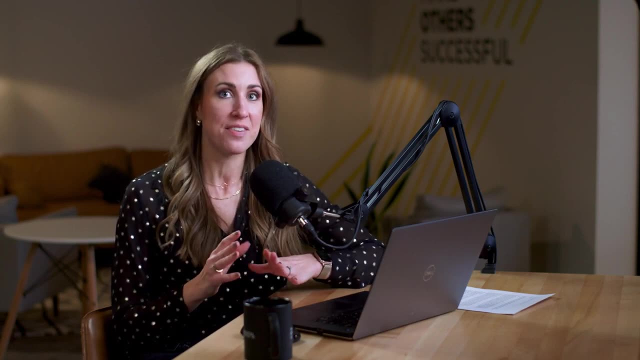 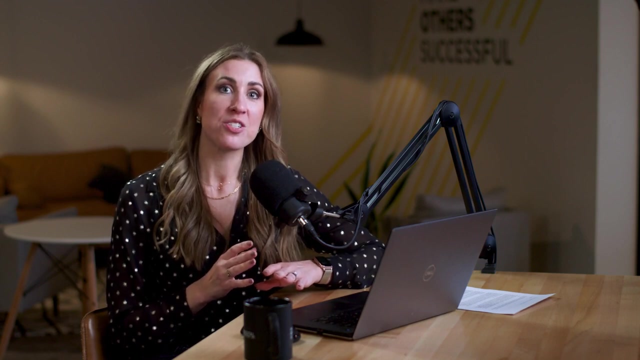 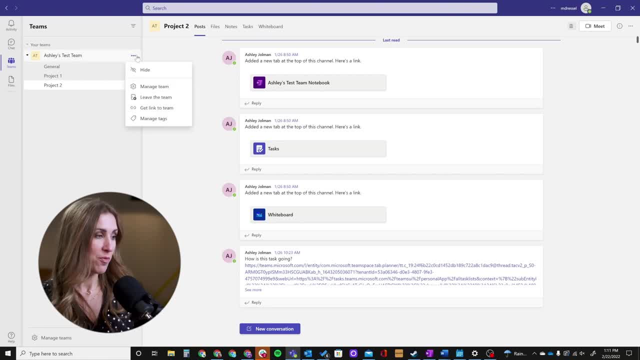 all of those integrated into your channel so that nobody has to do all the work that you're doing. So you can have all of those integrated into your channel so that nobody has to do all the work that you're doing. So you can have all of those integrated into your channel so that nobody has to do all the work that you're doing. So you can have. 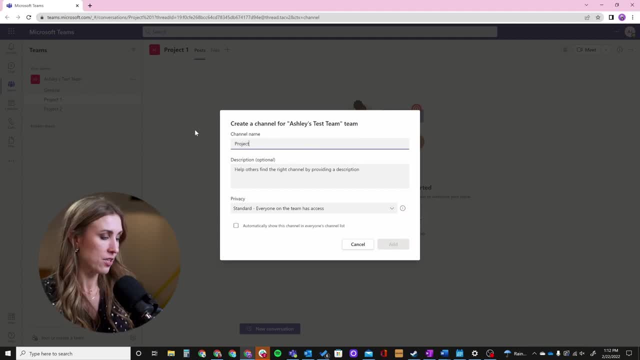 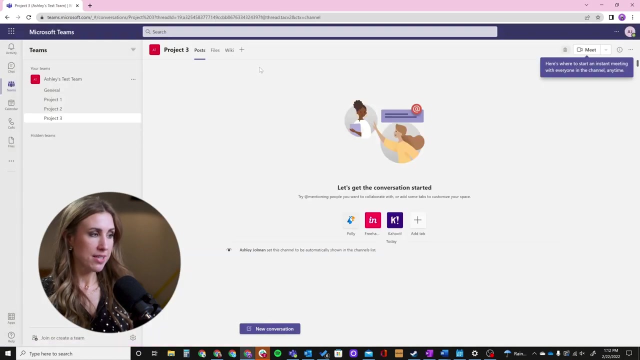 going to add a channel and I'm going to call this project three, so you can add your description and set the privacy which hopefully, for the sake of ease of this one, I'll just do standard to inherit the privacy settings for my team and go ahead and click Add and then it's going to show up. so a few things that 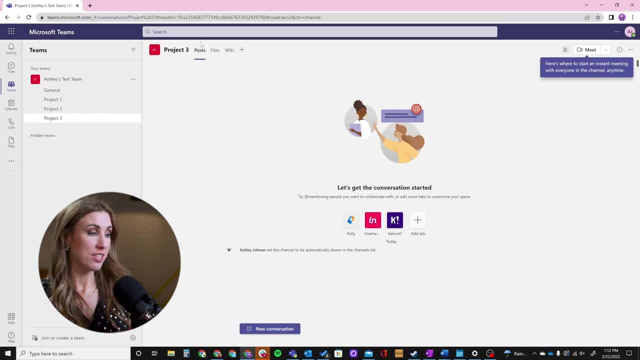 teams add ads. as standard are these tabs up here. so here's where you're really going to get into customizing how you're going to use this channel for your specific project. first, the posts tab that you'll always want to stay. I actually I don't think you even can delete it if you wanted to, but that's. 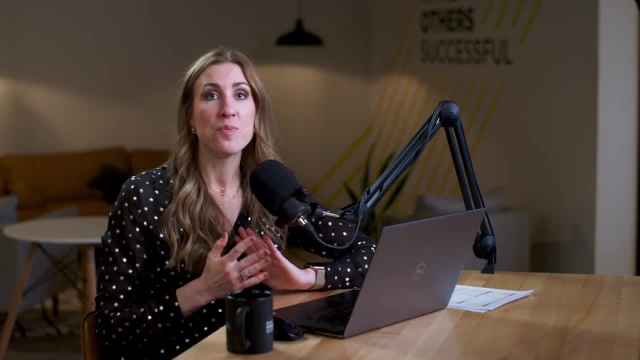 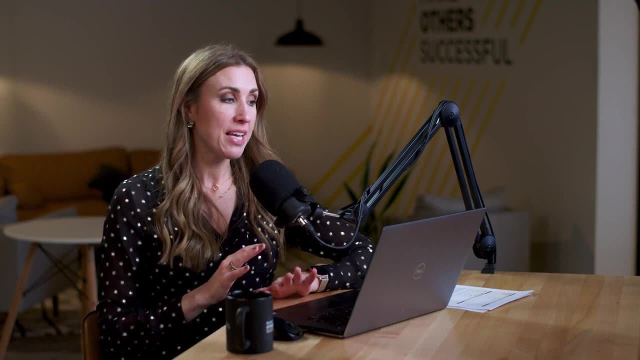 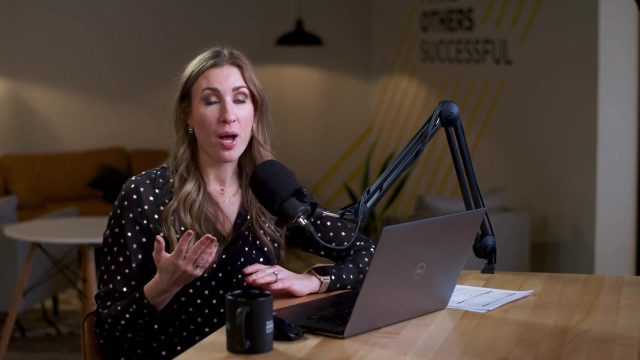 where all your communication is going to happen. so this is the hub of communication for your project. so we're not using email, we're not using phone calls, you know texting people. everything happens here and it provides transparency for your, for your project team. everyone knows, everyone's caught up. if communication occurs regarding the project, then the 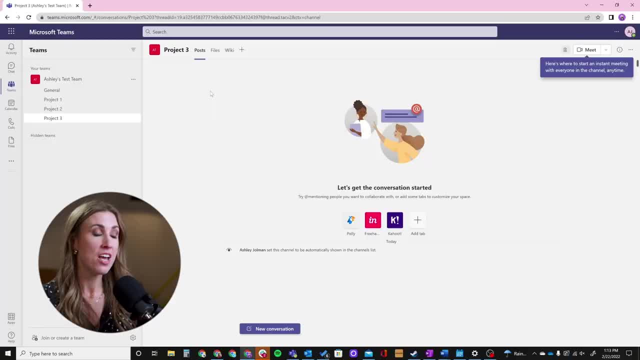 rest of the project team can see that and also be in the loop of what's going on. you can do conversations, you can create announcements. so, right here, start a new conversation. you can have quick chats with somebody from your project team. you can tag them. hey, I have a question. 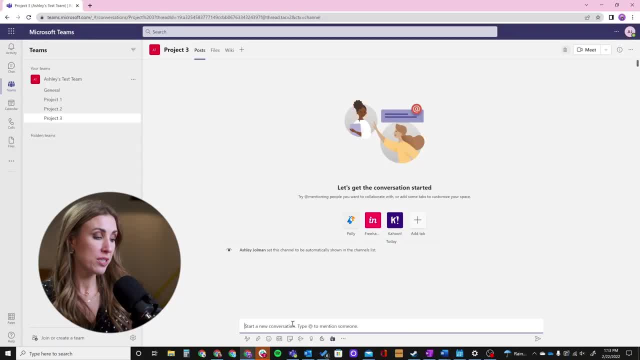 hey, this happened. this might impact your task or you can set up- if you're the project manager, you can set up an announcement just by clicking down here and again. these are features you may have already in teams, but it's just a powerful new twist when you're using them for a 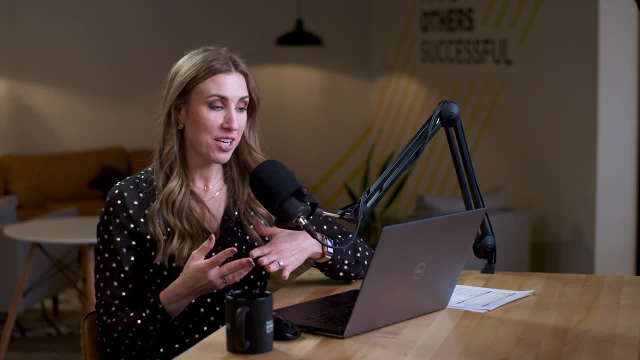 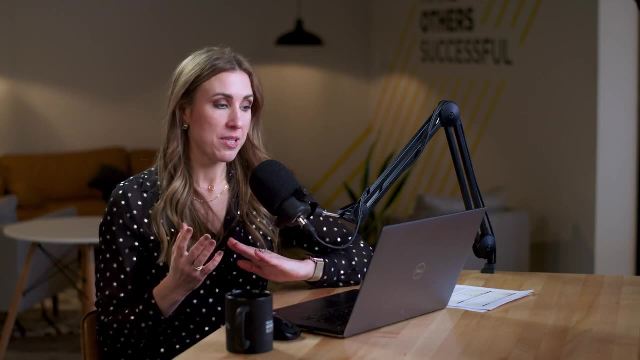 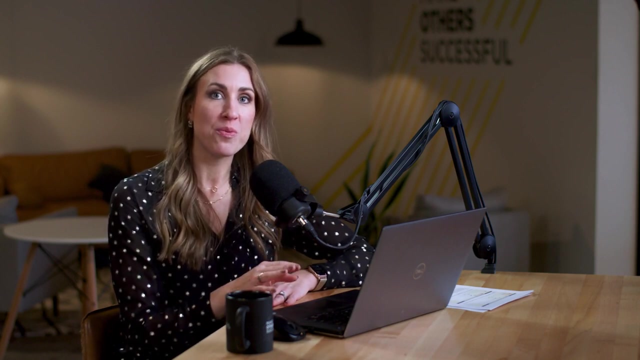 specific project so you can do your announcements here for a this change. I want everyone to know maybe there's a deadline update or just a status update in general, and the ability to have conversations, tag people, chat back and forth. is is really where the the power comes from in. 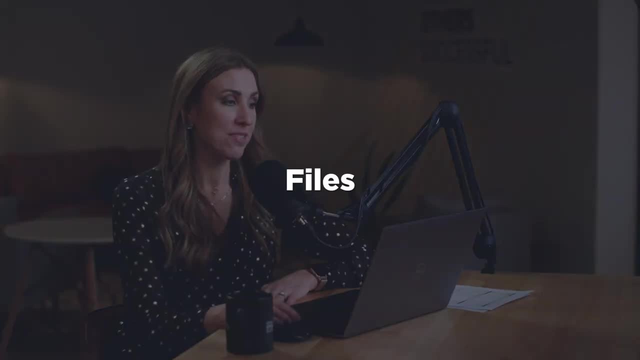 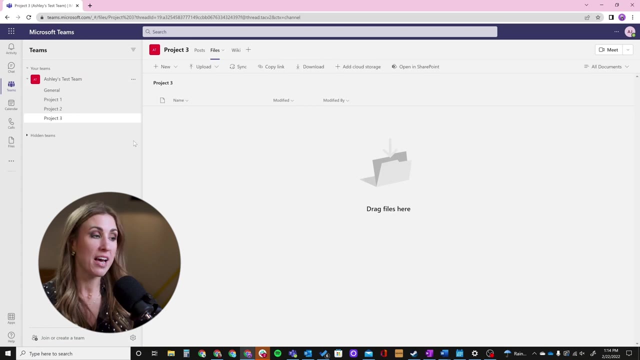 the post tab. the next tab that we'll go to is files. so every time you set up a new channel, you're also going to get a document repository and SharePoint that is associated. so that's why you'll see this here. you can open and open in. 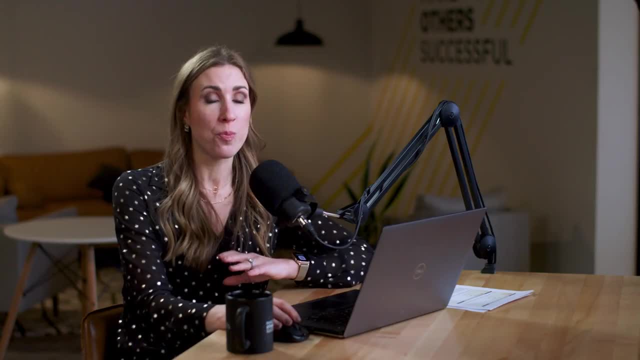 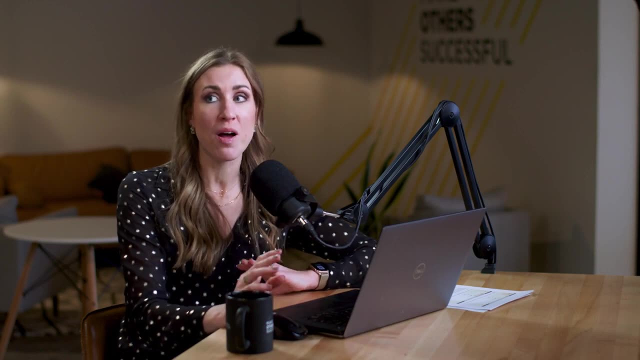 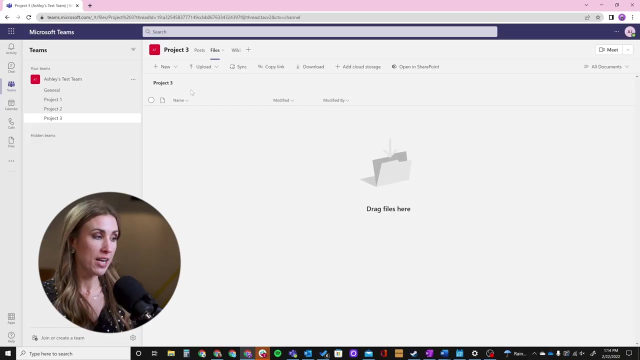 SharePoint, but that's going to give you a similar view. the point is, you don't have to leave teams to see all of the documents that are related to this project. so anything from PowerPoint, if you have a slide deck, if you have Word documents, Excel files, photos, you can organize those in this document library. 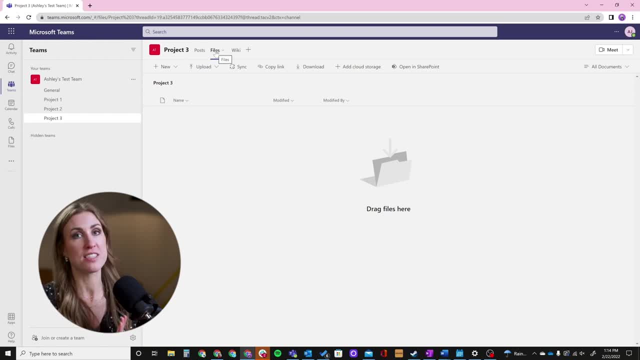 just by accessing the files tab, and everything for your project is going to stay right here. one of their benefits to this files tab is that you can take any of your documents in here and chat about them in the post tab. so, without having to open and save different versions of the files, I can post the document right. 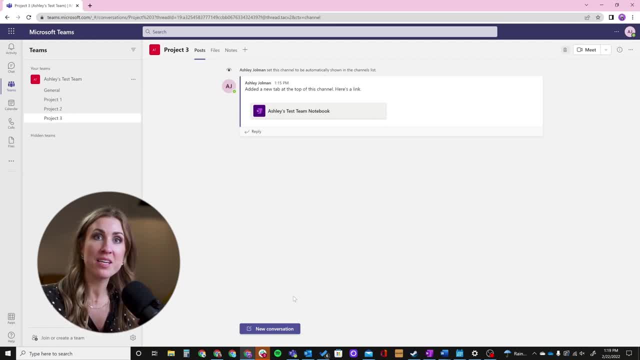 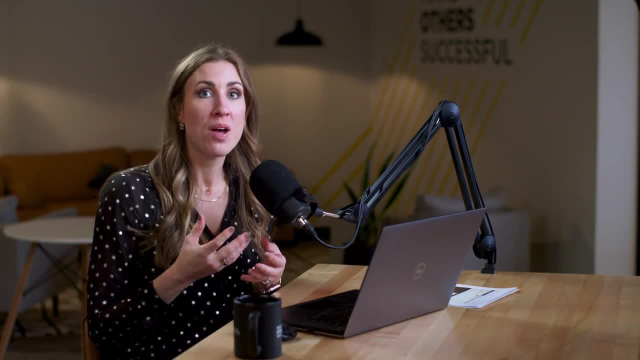 here and, you know, tag somebody on my project team, ask the person who's going to post the document and ask the person who's going to give their opinion. ask them to help me with it, and documents in the files tab will can be co-authored, so myself and anyone else, multiple people within my 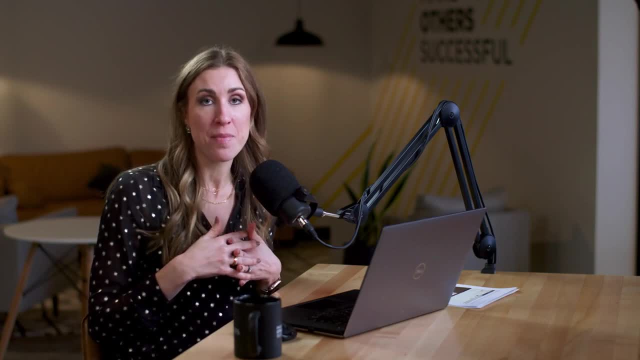 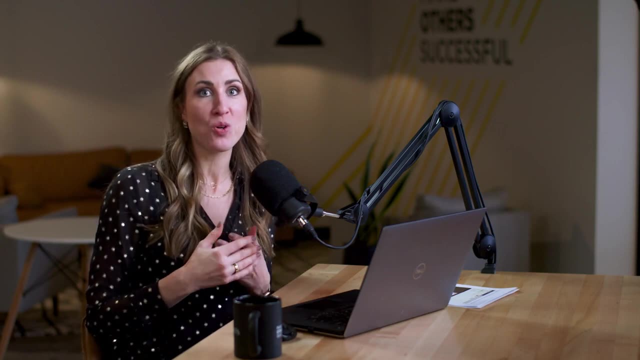 project team can work on a document together at the same time and there's no versioning issues because we're co-authoring live. nobody's emailing back and forth, nobody on the team has to wonder if they're using the most recent version, and then I can also ask for comments and feedback and in chat about. 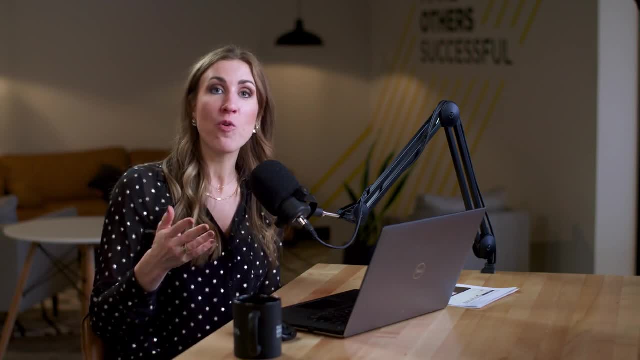 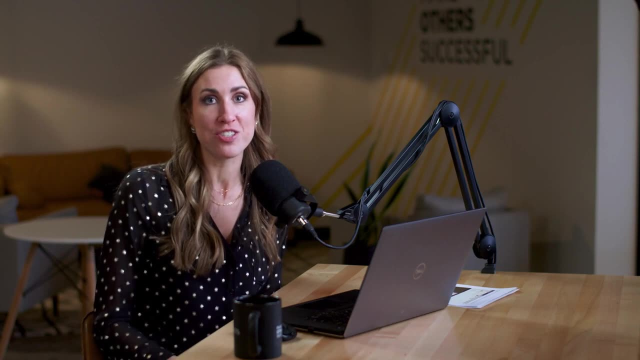 the document right here. and the other benefit, just like before, is that your whole project team is going to see discussions that you had about the document. So again, everyone's caught up without any additional steps. The next tab: I like to add a tab. 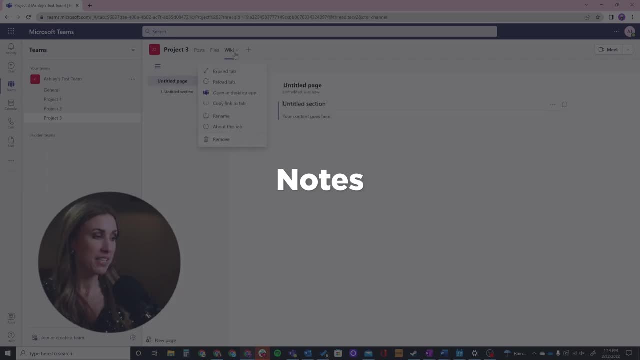 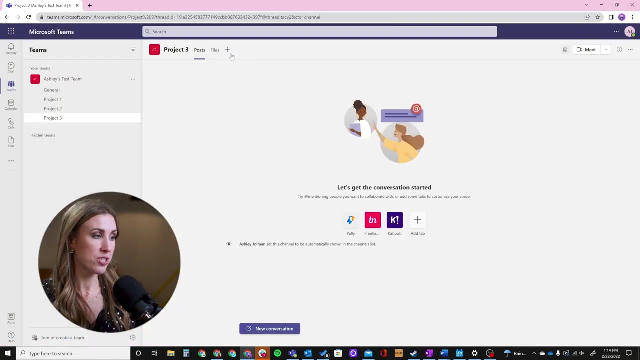 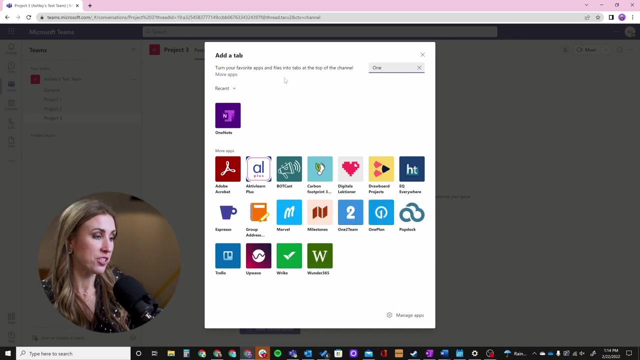 for notes. So Teams automatically gives you wiki. I'm going to remove that and just show what we like to use it for, which is OneNote. So again, as long as you're using something in the Microsoft 365 suite, it's going to inherit the permissions of your team. So when I add a OneNote, it's going. 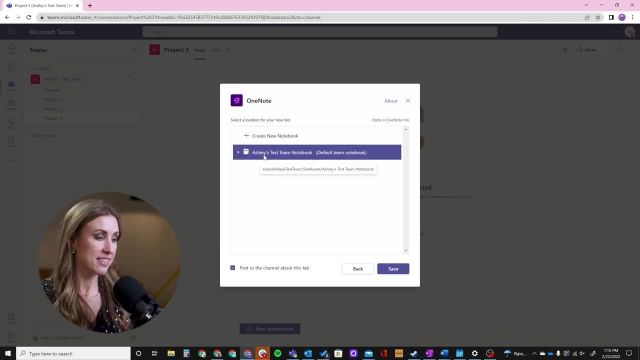 to use the same security settings that my team already has set up. There was a team notebook automatically created when I created this team, So I'm just going to select that I do want to post to the channel, just because I want everyone on my project team to know where we're going to. 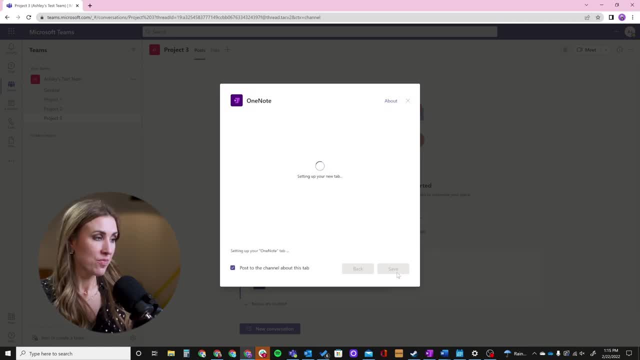 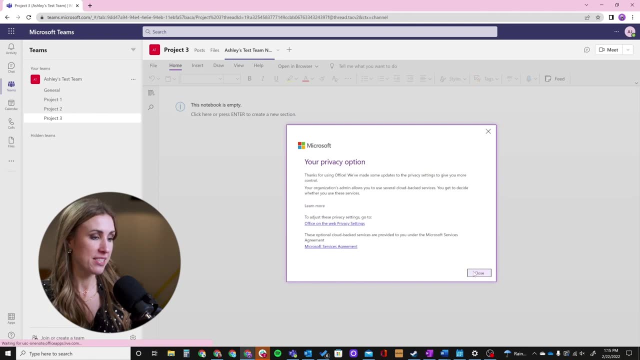 be going for notes And then I'll hit save And then you can see how that will show up. It shows up Ashley's test team notebook. I'm going to go ahead and rename this Close out of that And I'll. 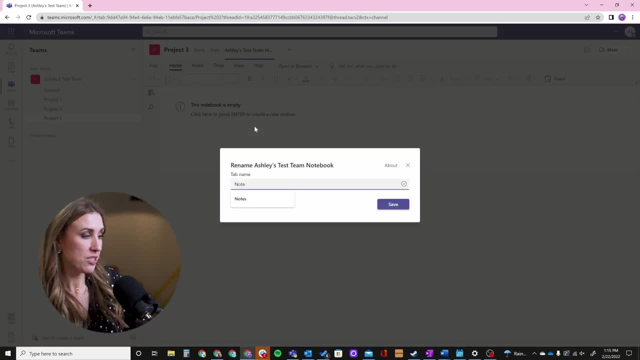 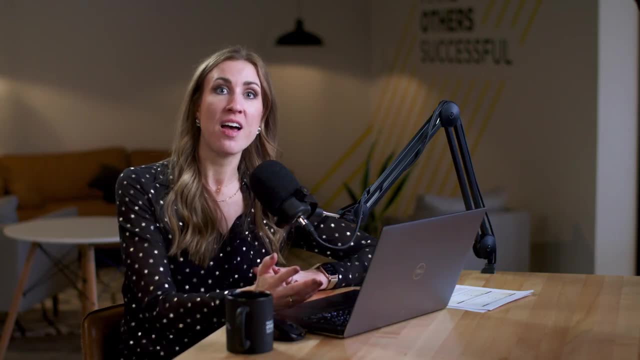 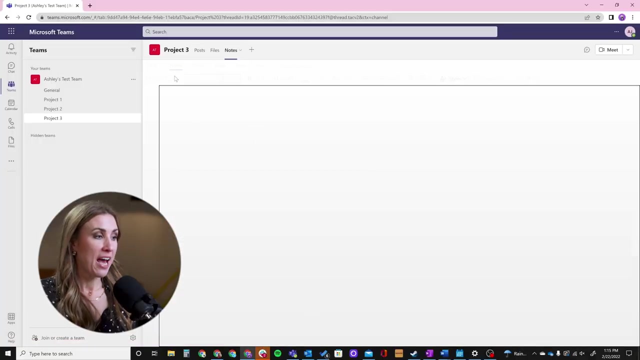 just rename it to something simple which is notes, Because, again, it doesn't matter what tool you're using. You can keep wiki in here. You can use a different tool for your notes. As long as that tab is called notes. your whole team knows where to go to access the notes. So here you can. 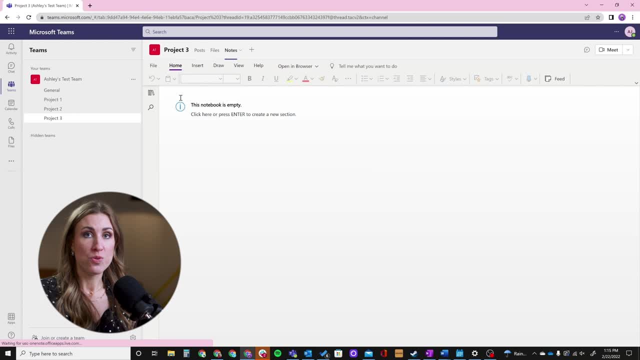 have anything from meeting minutes to notes or documentation about your project, And then there's never a question from your project team where they can access that information. So if somebody missed a meeting, they know right within the channel. they can just go to notes. 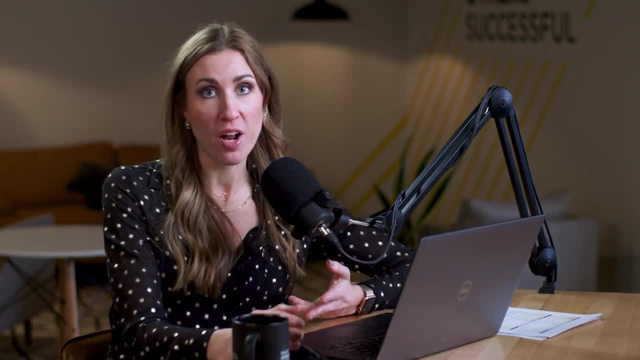 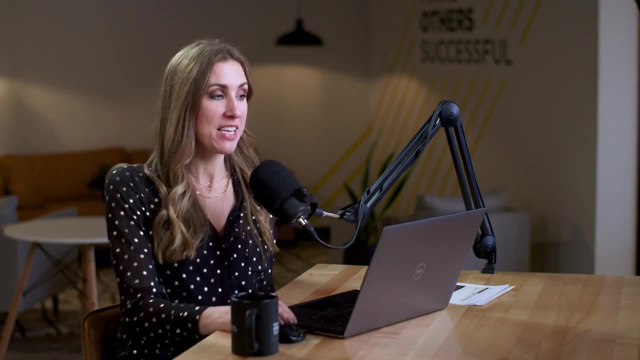 look at that day's meeting minutes that they missed and be all caught up without having to ask anybody where things are. The other tab that I always like to make sure is added to my project is a tab, for I'll call it task management. So whichever tool that you are using to assign and 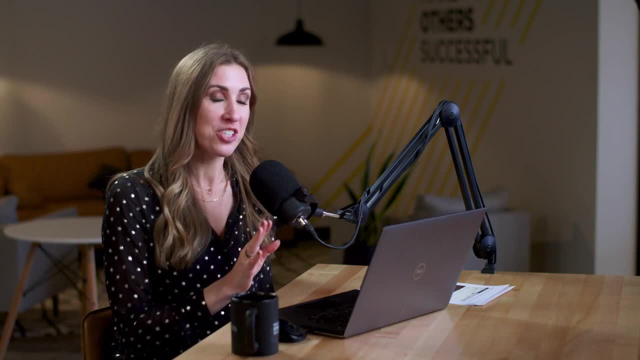 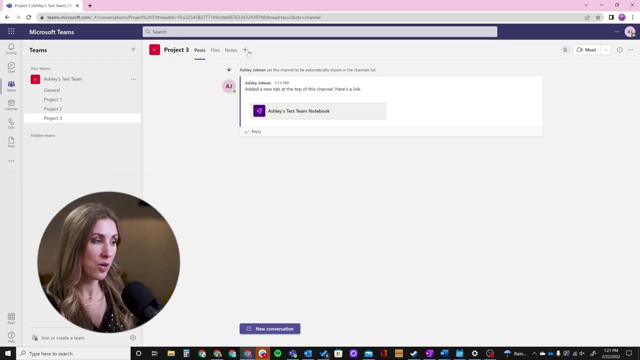 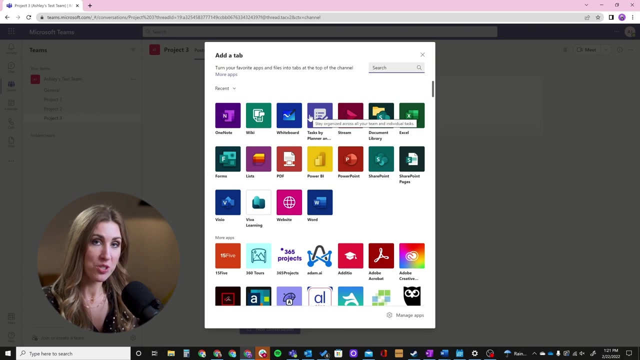 track tasks in your projects. make sure it's added for really the best practice for project management in Microsoft Teams. So the benefit here when you add a tab is that Teams integrates with a lot of different project management tools. So you do have your Microsoft ones project planner, but there's other ones in. 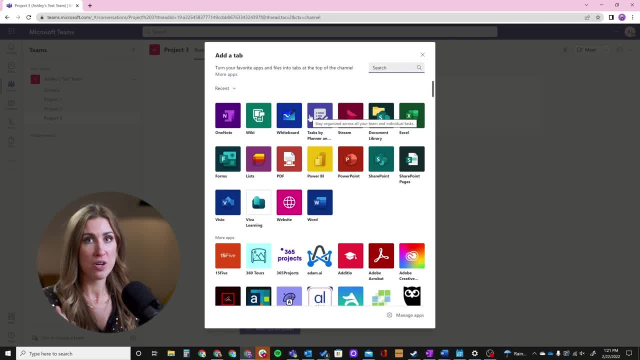 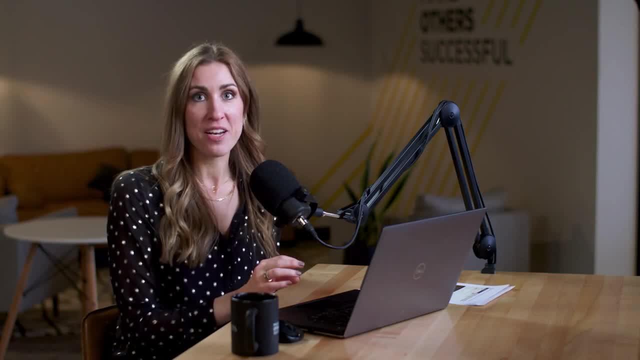 here too, If you use a third party, if you use mondaycom, Trello, one of those other tools, if that works best for your project, you can add that as a tab and you're still getting the benefit of having your central source of truth, which is all the aspects. 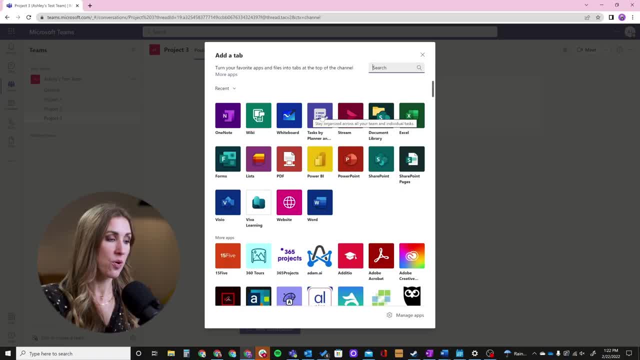 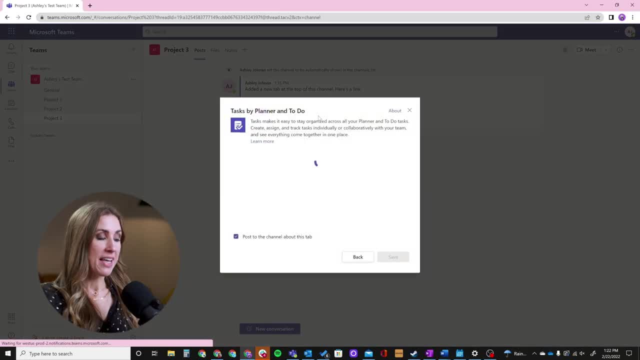 of your project in one place. I'm going to use planner- So that's what's called tasks by planner- and to do as this app right here And again. the benefit of using a Microsoft tool for task management is that it's going to inherit the permissions that you've already created for. 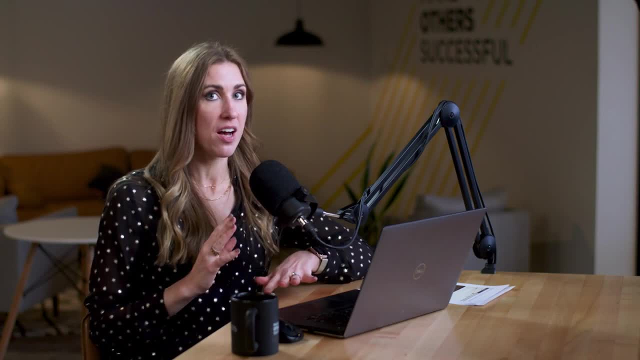 your team, So you don't need to. there's no other logins, logouts, setting up, security, all of that. You can create a new task management tool and you can add that to your project. So that's what I'm. 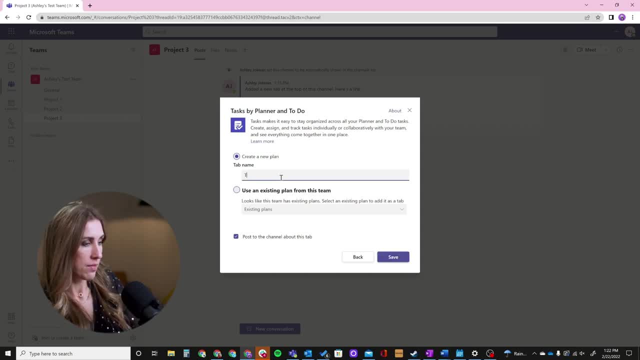 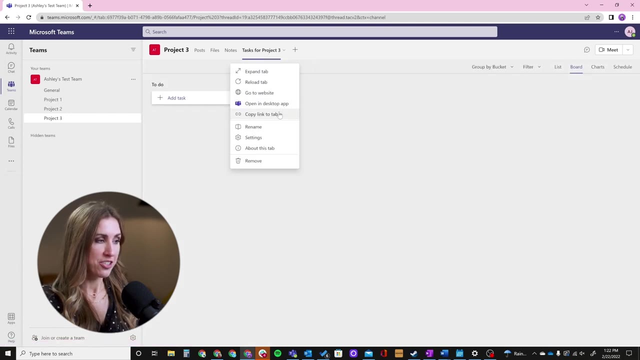 going to do So. I'm going to create a new plan, So I'm going to call this: yeah, tasks for project three. And then again you can post to the channel about this tab, just to keep everyone informed, And I'll rename this tab again, just like we did with the notes one. I'm just going to rename this. 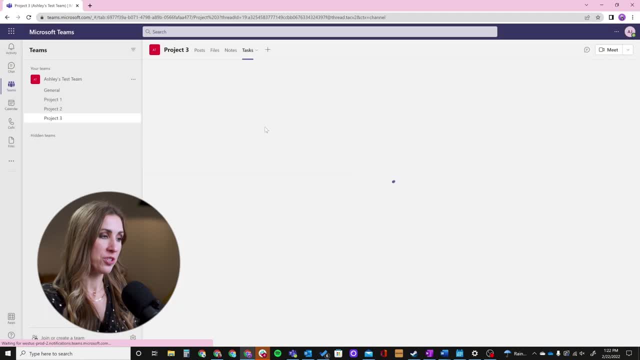 to tasks, because it doesn't matter which tool you're using. It just matters that people can quickly and easily access what they need. And now I'm going to go ahead and create a new task. So now tasks you can. you're going to have a planner board that's really integrated directly. 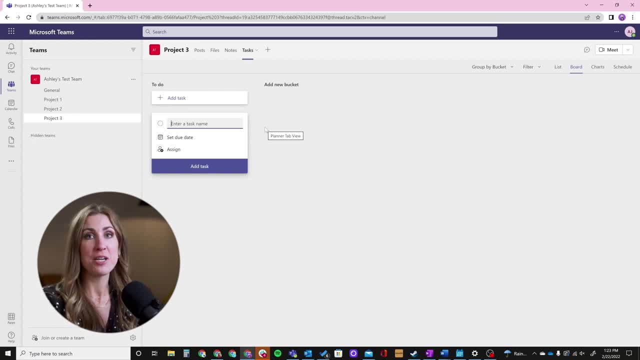 into your channel. So here's where you can add your tasks, make sure everything's assigned to people, And then you can have discussions and remind people about tasks all within this channel, And again, without ever having to leave. Here's where you can also get into your charts for status. 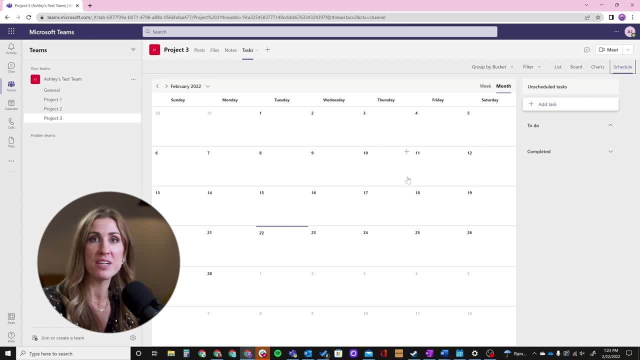 updates for schedules, If anyone on the project team wants to view the calendar or see where the project is at, And then you can also add your tasks to your channel. So here's where you can add your tasks And again, without ever having to leave, Here's where you can add your tasks to your channel. 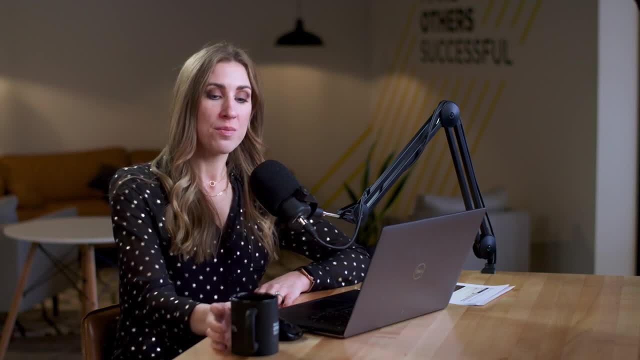 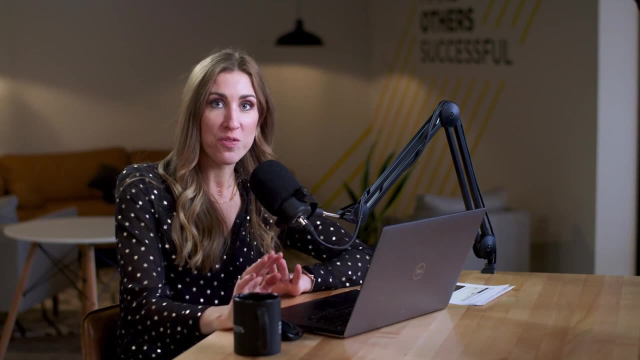 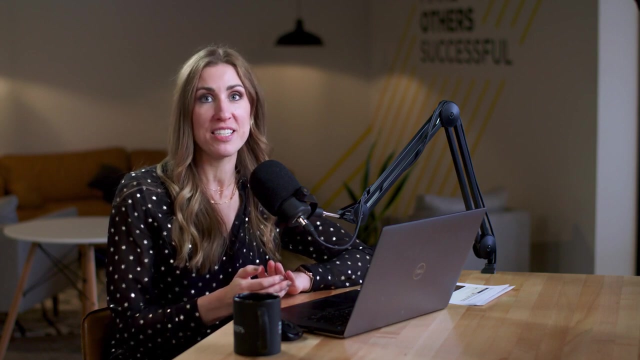 And this eliminates the question that people always raise, which is: I don't know, how do I see what's assigned to me? How do I find out what my due dates are? This solves all of those problems that project managers can run into, because there's one central source that your whole team knows: they 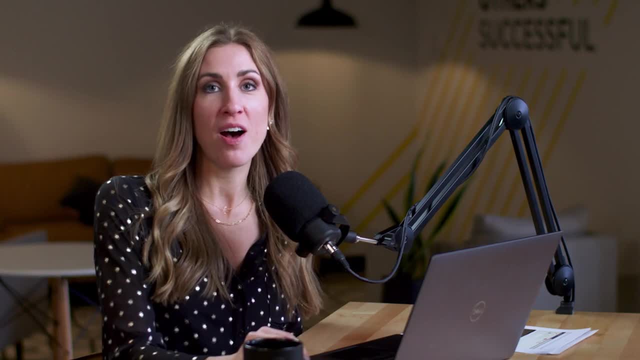 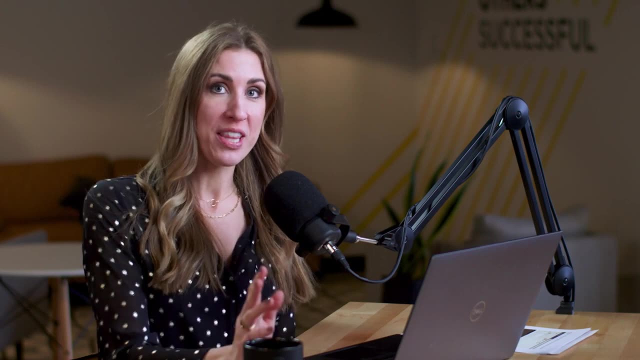 need to access to get all of that information. And finally, just one last note is that anytime you're setting up a project in Teams, you can continue to add tabs, the way that we just did for the notes and for the tasks, And so that's where you can add your tasks to your channel. 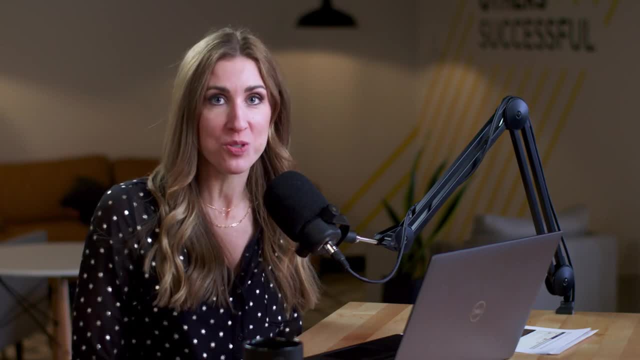 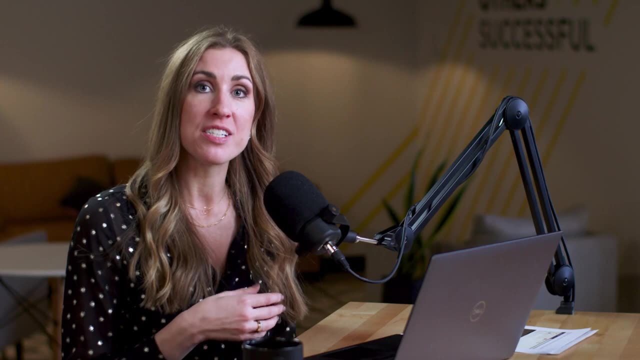 If there's any tool that's relevant to your specific project, whether that be a whiteboard tool, if that's how your team generates and collaborates on ideas- maybe there's a design site, depending again on what type of project and what tools your project team likes to use. 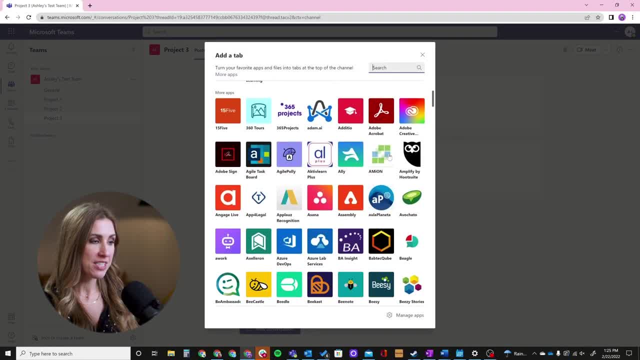 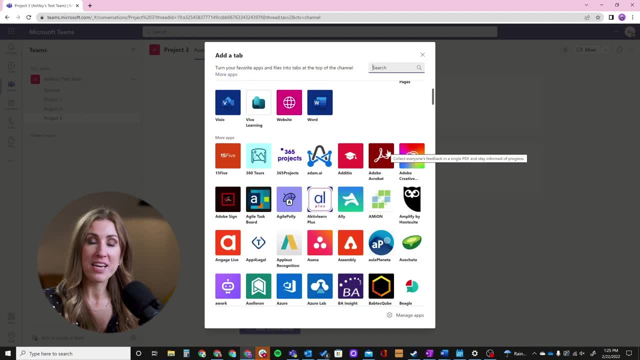 Teams integrates with so many different applications that you can scroll through and add all of those things as a tab. Or if it's just a website, you can just add a website also to add as a tab, And that way you're just keeping track of what's going on And then you can add all of those things as a 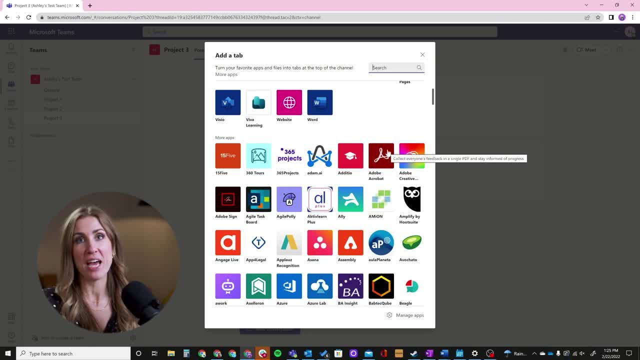 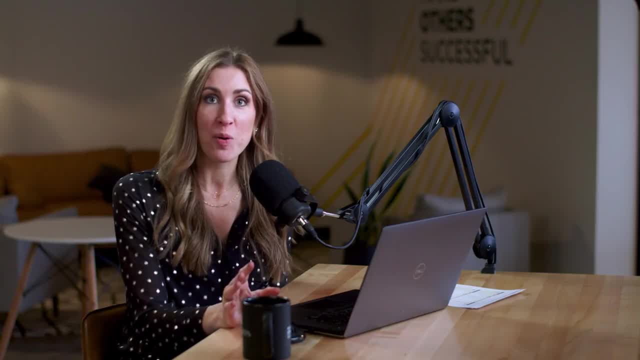 project, keeping with the consistency of team members only having to access the channel to get to anything they need for the project. Teams is highly customizable And you're going to be able to set up a project in a way that works best for your specific team and project. Now that we've 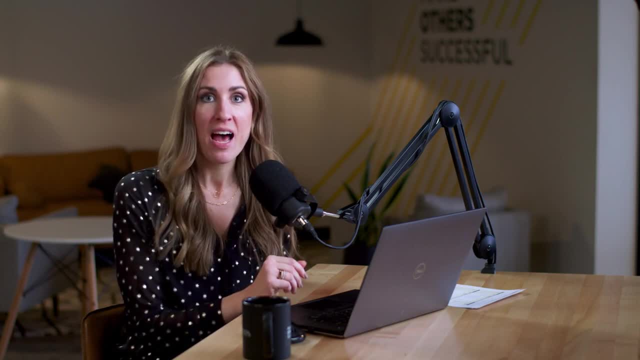 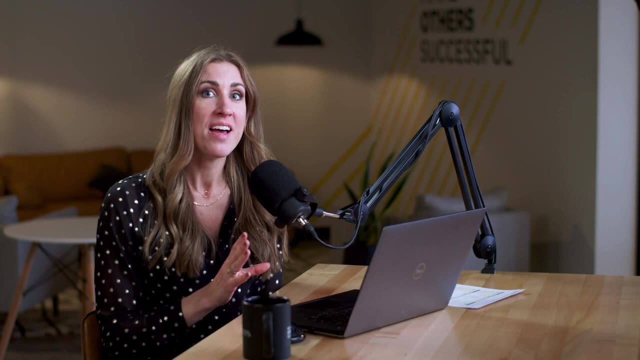 gone through the setup of an example project in Teams. how can we use this for future projects? If I've found what I like, this is what works well for us. My team is used to it. You can actually save yourself a lot of time if you're a project manager, And if you're a project manager, you can. 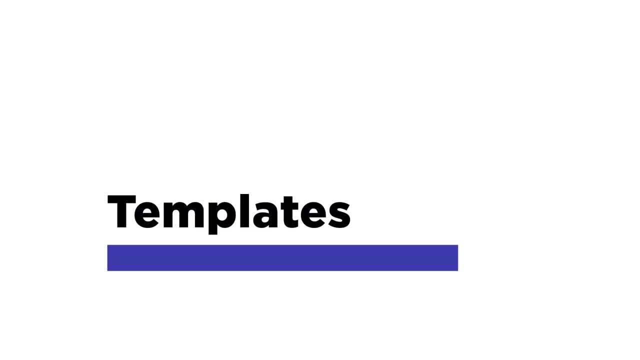 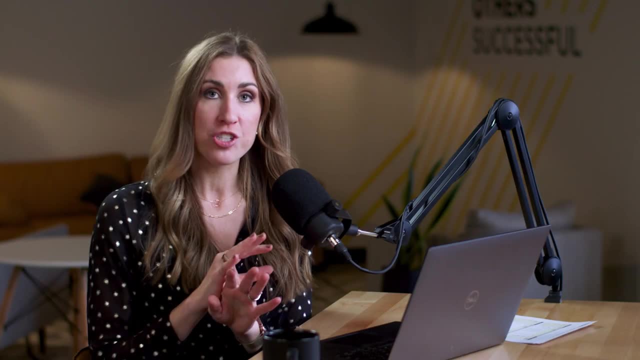 save yourself a lot of time by using your project setup as a template. We actually have a whole other video on this. if you want step-by-step instructions on how to use a current channel setup that you like as a template, And what that'll do is next time you create. if I were to start project.